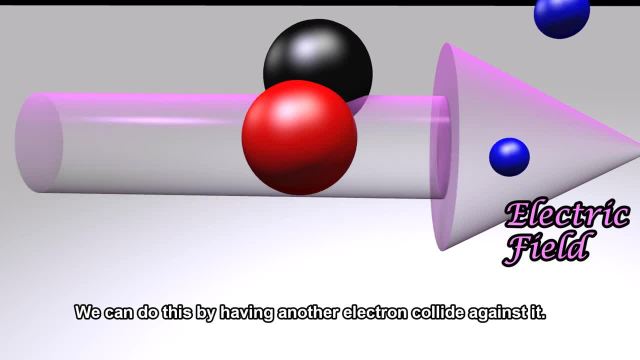 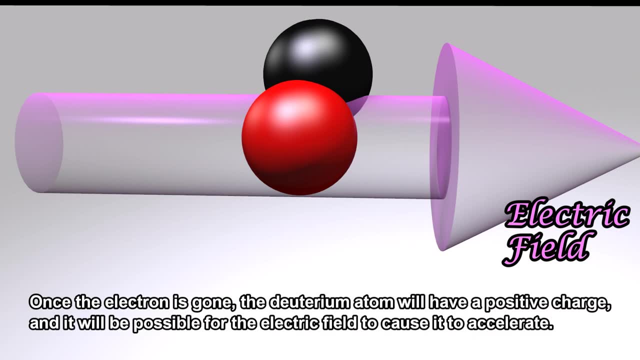 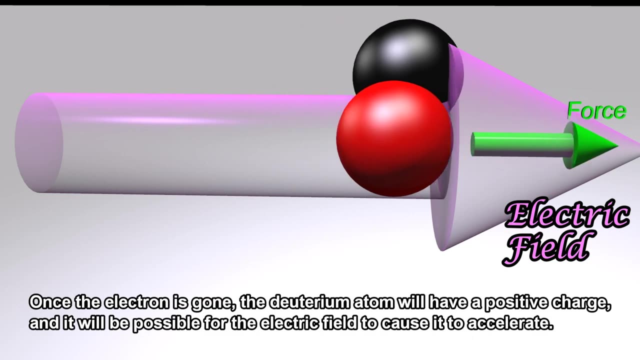 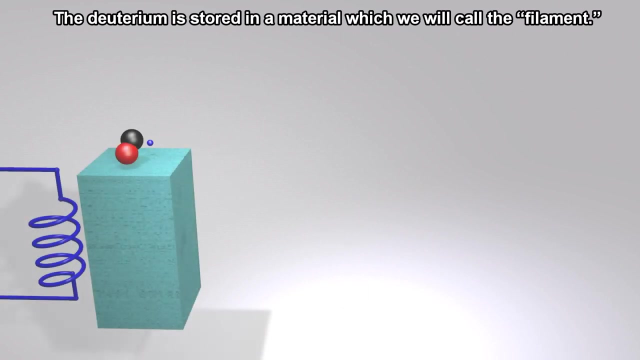 We can do this by having another electron collide against it. Once the electron is gone, the deuterium atom will have a positive charge and it will be possible for the electric field to cause it to accelerate. The deuterium is stored in a material which we will call the filament. 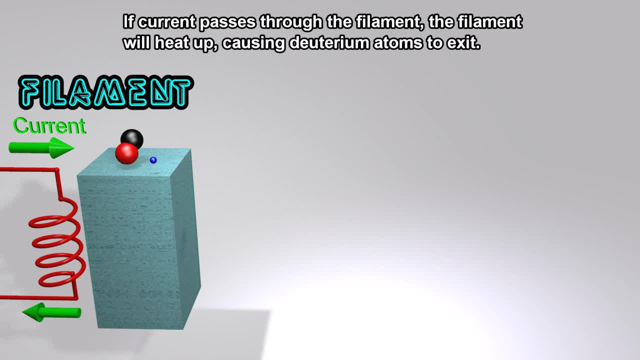 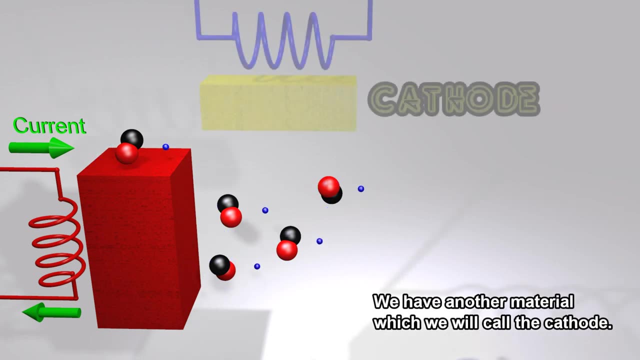 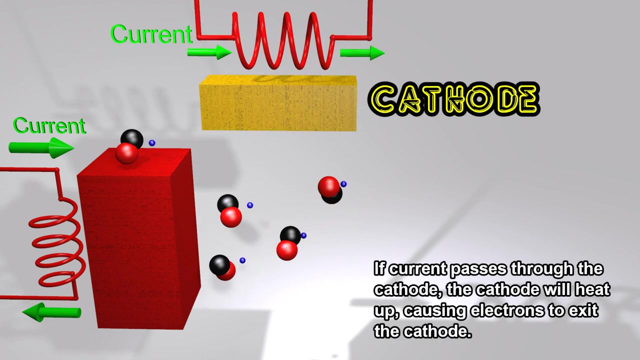 If current passes through the filament, the filament will heat up, causing deuterium atoms to exit. We have another material which we will call the cathode. If current passes through the cathode, the cathode will heat up, causing electrons to exit the cathode. 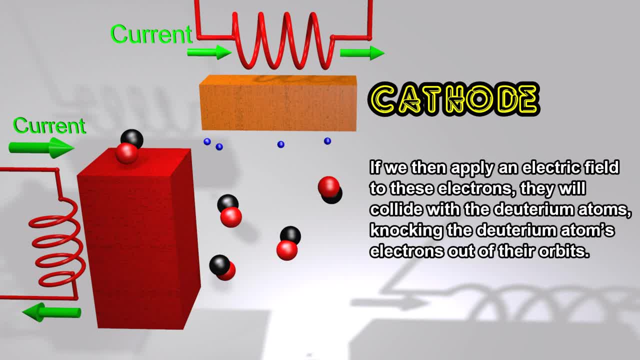 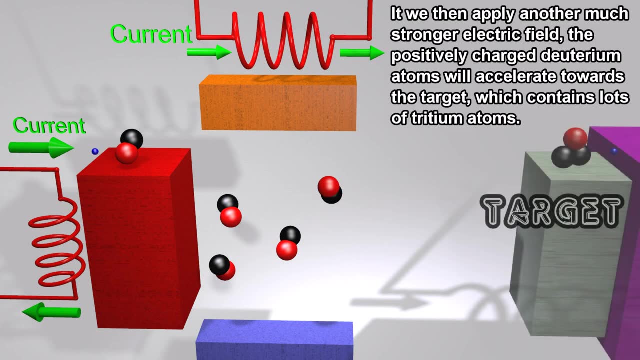 If we then apply an electric field to these electrons, they will collide with the deuterium atoms, knocking the deuterium atoms electrons out of their orbits. If we then apply another, much stronger electric field, the positively charged deuterium atoms will accelerate towards the target. 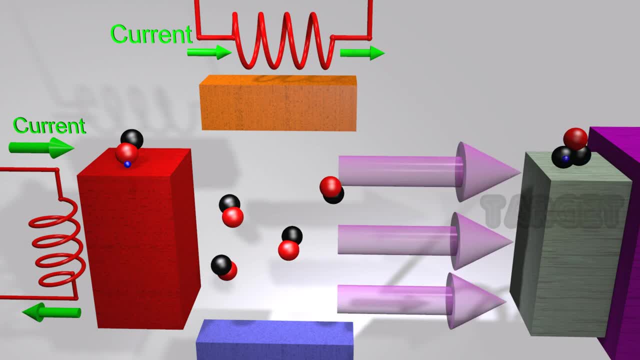 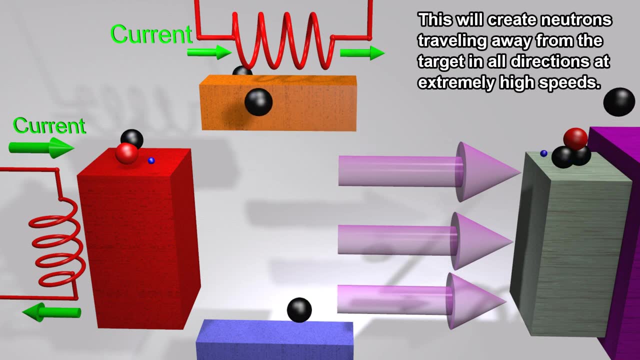 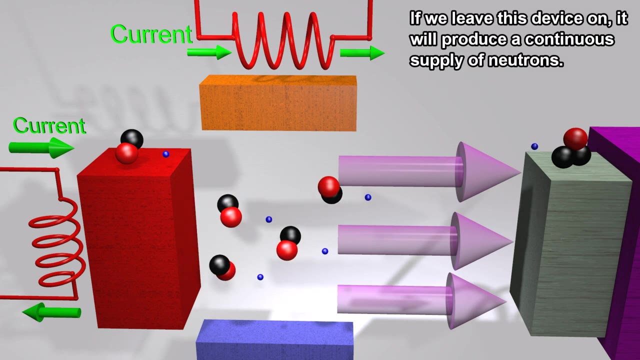 which contains lots of tritium atoms. This will create neutrons traveling away from the target in all directions at extremely high speeds. If we leave this device on, it will produce a continuous supply of neutrons. We can control the rate at which neutrons are produced. 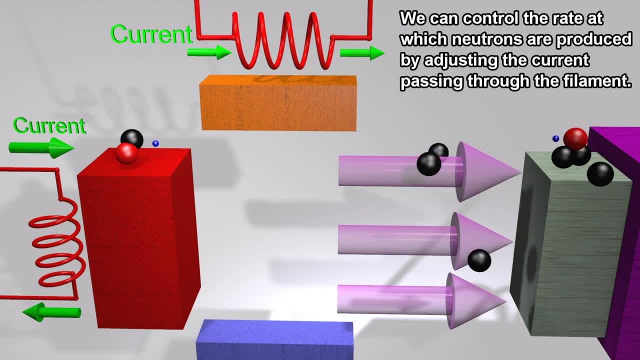 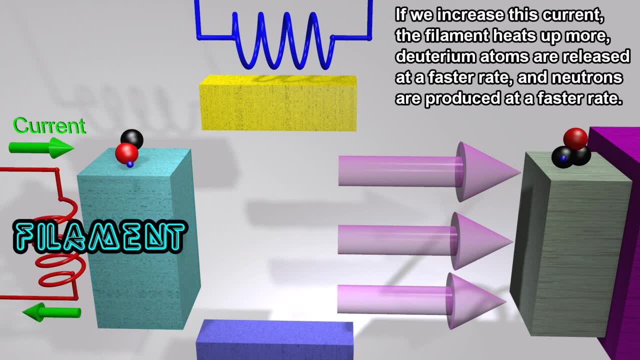 by adjusting the current passing through the filament. If we increase this current, the filament heats up more, deuterium atoms are released at a faster rate and neutrons are produced at a faster rate. The filament current and the cathode current are just for creating heat. 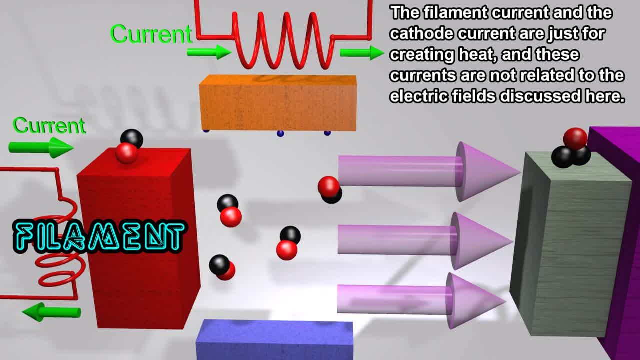 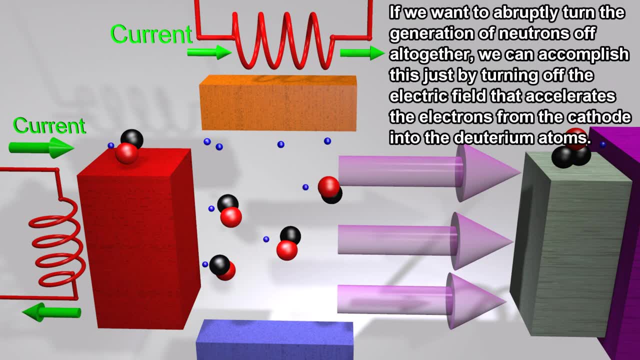 and these currents are not related to the electric fields discussed here. If we want to abruptly turn the generation of neutrons off altogether, we can accomplish this just by turning off the electric field that accelerates the electrons from the cathode into the deuterium atoms.